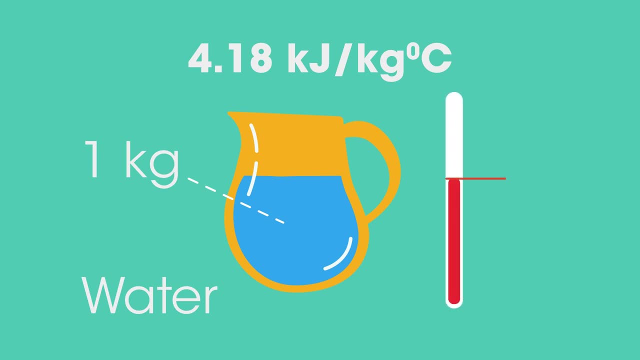 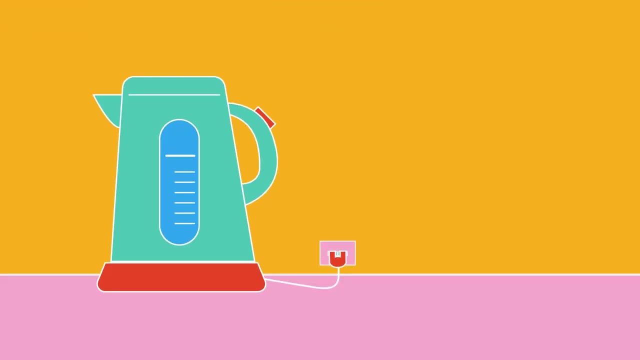 Celsius. This means it needs 4.18 kilojoules to heat one kilogram up by one degree Celsius. We can use the equation Delta E equals MC, delta theta to work out the energy needed to boil a kettle of water If we take 0.5. 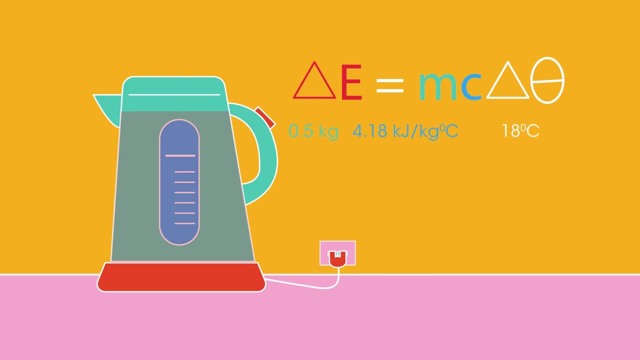 kilograms of water or half a liter at 18 degrees Celsius and heat it to boiling or 100 degrees Celsius, then energy used equals 0.5 times 4.18 times 82, which equals 171.2.. This assumes that there is no loss of energy during heating, which of course there will be. 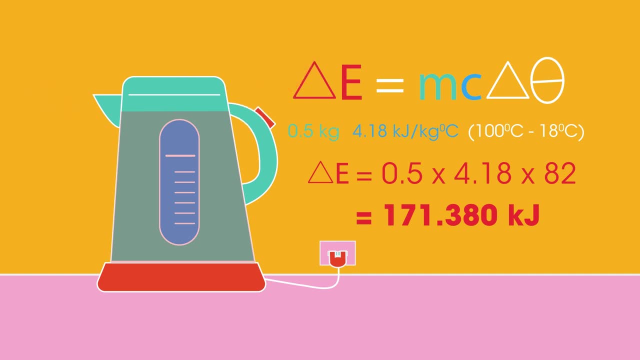 Heat and sound will be lost to the surroundings. If this kettle took 80 seconds to boil, then we can begin to estimate the power of the kettle. Power is the rate at which energy is transferred. Power equals energy over time, So we get 171.38 kilojoules. 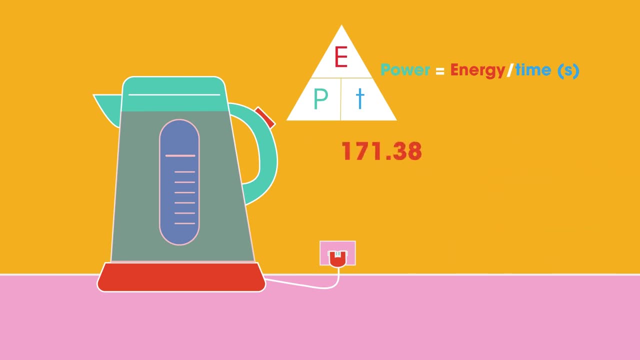 This is the temperature of the kettle orופ. the 7.omos per liter given by the상 Tropical Thermitez and a took on 37 times before. So this� 3.38 over 80 equals 2.14 kilojoules per second, or 2.14 kilowatts. 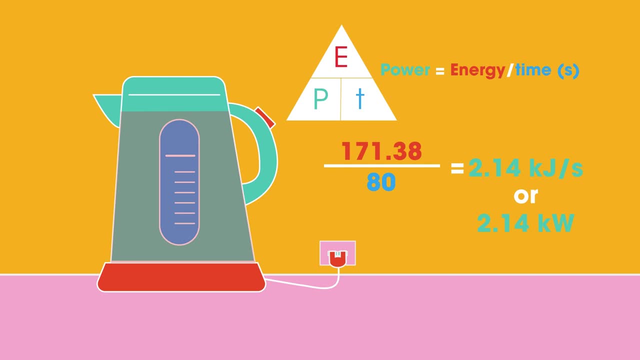 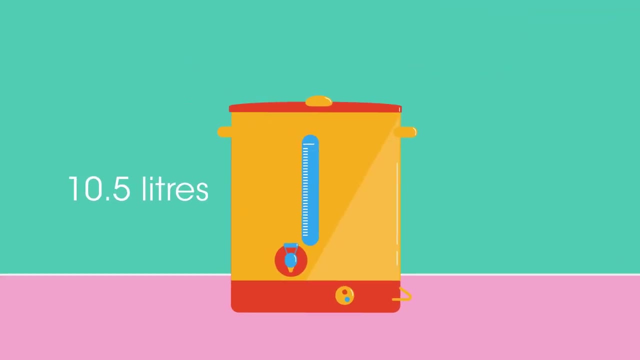 This answer will be slightly lower than the actual power due to the kettle being uninsulated. This water boiler holds 10.5 litres of water. How much energy is transferred if the water at 14°C is heated to boiling point? Pause the video while you work it out. 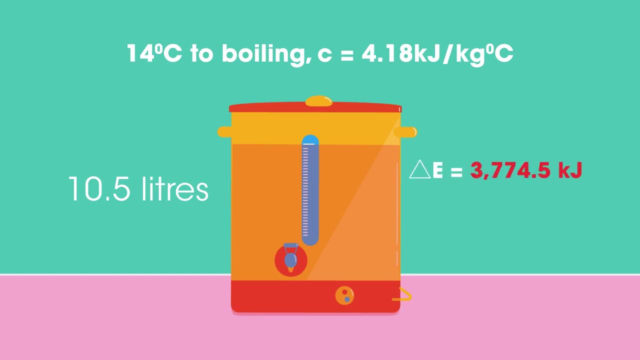 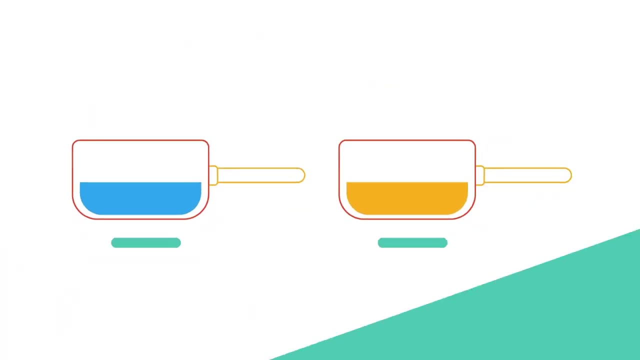 Did you get 3,774.5 kilojoules or 3.775 megajoules? Different materials have their own specific heat capacity. This has consequences in our everyday life that we may not be aware of. Most of us probably cook with water more often than we do with oil. 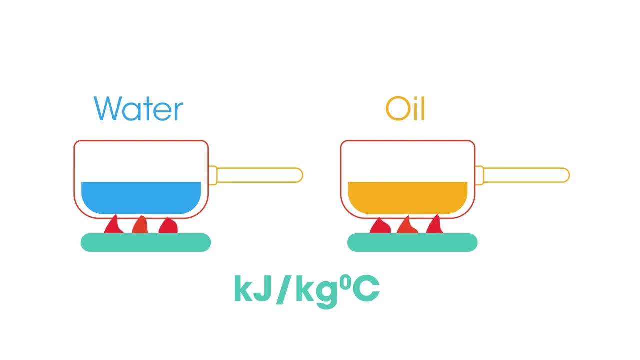 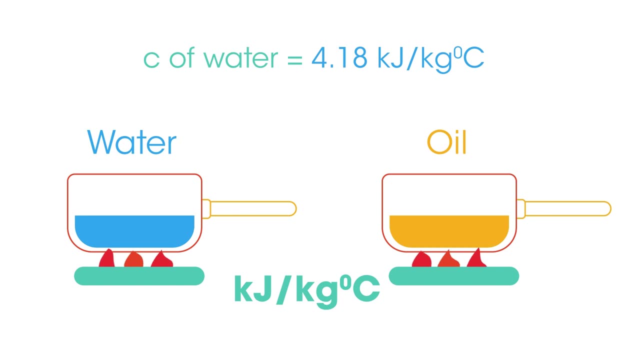 Imagine that we are here. We are heating pans of water and oil over identical heat sources. Specific heat capacity of water is 4.18 kilojoules per kilogram per degree Celsius And specific heat capacity of olive oil is 1.97 kilojoules per kilogram per degree Celsius.